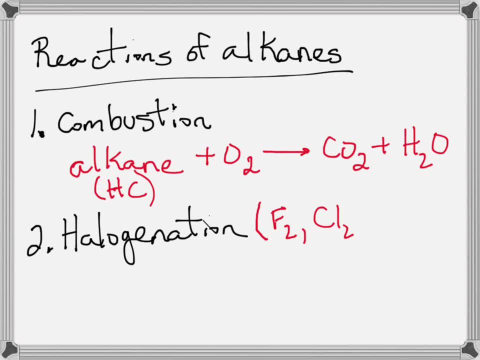 remember these are all diatomic molecules, meaning there's two of them, so it's F2, meaning there's two fluorines to make. the molecule F does not exist by itself in nature, it only exists as two of them together. Chlorine is the same as like bromine and iodine. 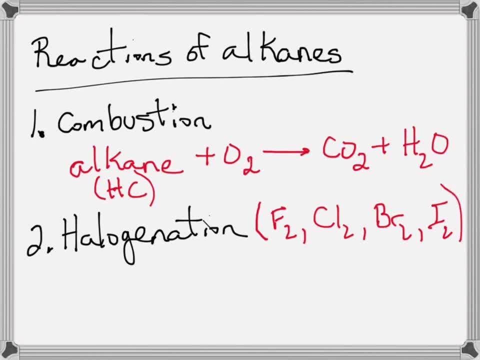 And if you look on the periodic table, they're all in the same column And so therefore they're very similar in reactivity And so those are halogens. So halogenation is putting these on an alkane. So, again, if I give you an example- and I'll just use something very simple just to start- 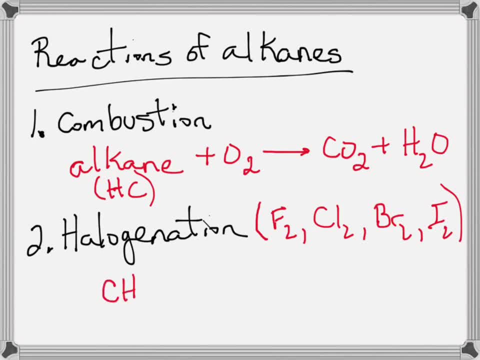 but it could be any alkane. If you have an alkane like methane, CH4, that's an alkane And we add a halogen and we can use any of them. I'll just use fluorine as an example. This reacts. if you give it a little bit of heat, this reacts. 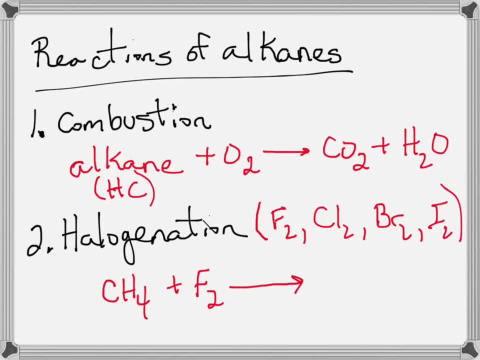 And one of the fluorines will switch spots with one of the hydrogens on methane, And so if we switch spots, we'll remove one of the hydrogens- that's CH3, and replace it with the fluorine. So there's CH3F plus and we used to have two fluorines. 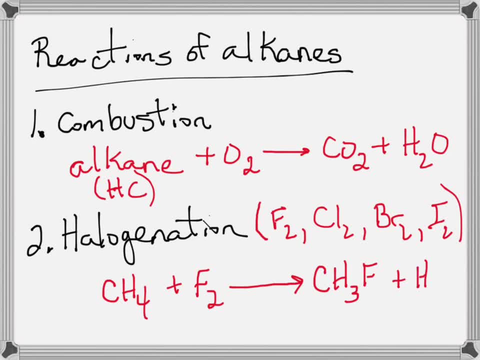 they have to be in the same column And there is a reactant, but now we're going to have an H has replaced one of the Fs, And so now we have HF And if you give it enough fluorine into this reaction, if you get a lot of fluorine in. 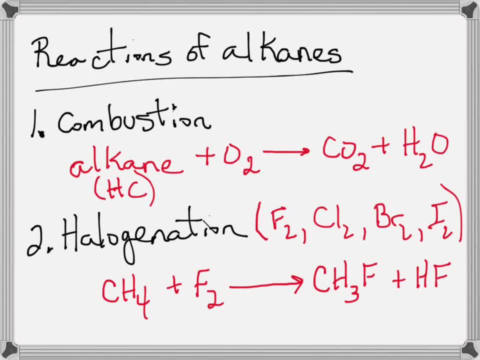 the reaction, all the hydrogens on the carbon can be removed and replaced with fluorine. So if you let this reaction continue and keep adding fluorine, you'd eventually get to the point where you're CH or CF4, if you could just keep putting fluorines in place of hydrogens. 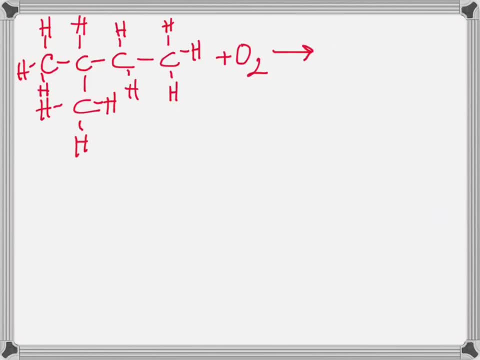 So why don't you give it a try? Here is a reaction of these two, of this reaction right here. Go ahead and pause the video and write down what the products are and then come on back and we'll talk about it. So in this video, in this reaction, we can see that this molecule over here, this big 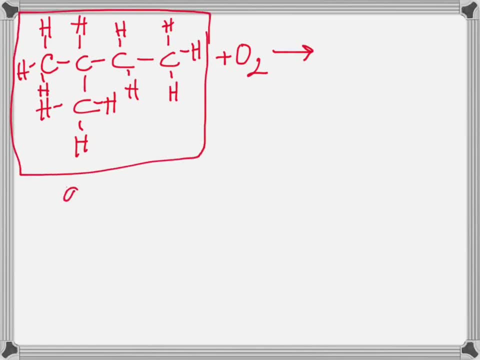 molecule right there, That's an alkane, And if we oxidize it by adding oxygen, this is a combustion reaction. So the products of this are simply CO2 and water. This is a combustion reaction And notice: the products here are always going to be the same for a combustion reaction. 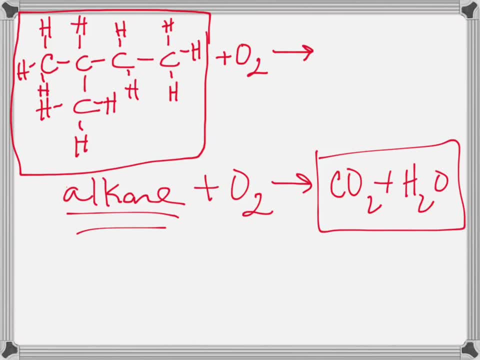 It doesn't matter what alkane you start with, Notice we have in the alkane carbons and hydrogens. We have an oxygen, We have an oxygen out here And notice in our products we didn't lose any of those. I still have carbons, oxygens and hydrogens. 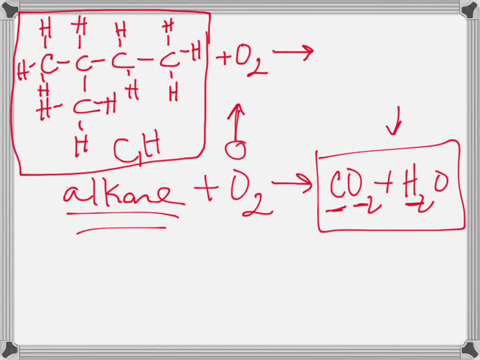 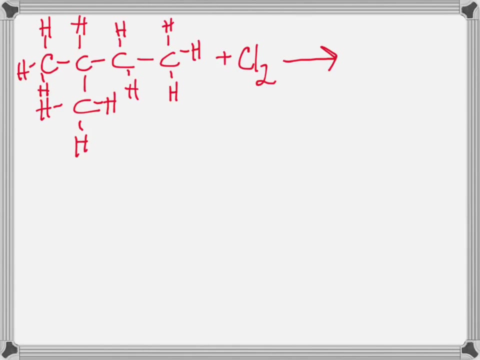 Again, this reaction is not balanced, but nonetheless there are our products, So it doesn't matter how big and complex the alkane is, the products are always the same in a combustion reaction. So now here's another reaction. Go ahead and pause the video. 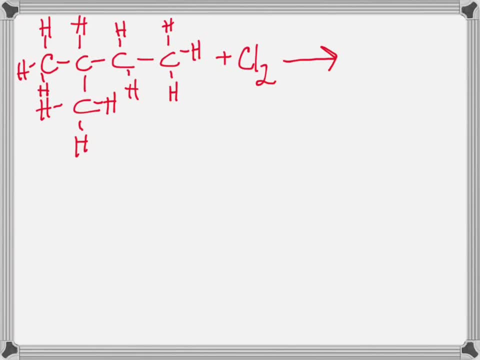 Determine what the products are. Once you think you've got them, come on back and we'll chat about it. So, again, the first thing you have to do is identify what reaction this is, and this is a halogenation reaction. Notice we have an alkane, our same alkane we had in the previous reaction. 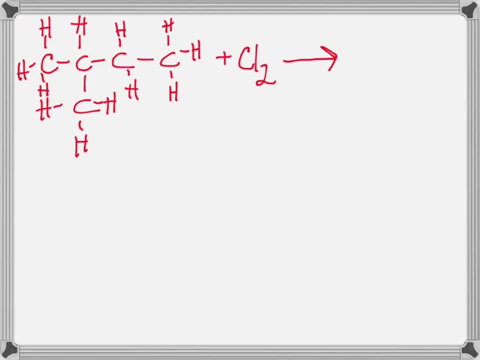 So we have an alkane and then we have a halogen. So this is going to be a halogenation reaction, which means basically, one of the chlorines is going to switch places with one of the hydrogens, and we have a lot of hydrogens. 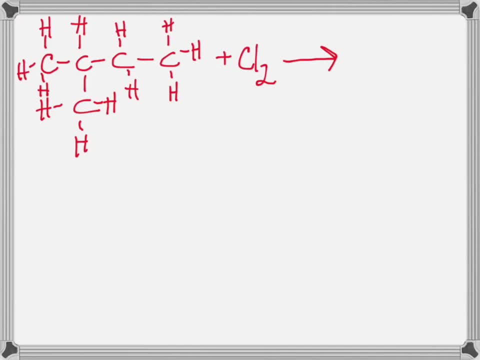 to choose from, And so in this case, you can pretty much choose any one you want, and that's a potential product. Now, some of the hydrogens are more likely to change spots with the chlorine, but for our argument at this point, let's just say all of them are possible, and so, therefore, 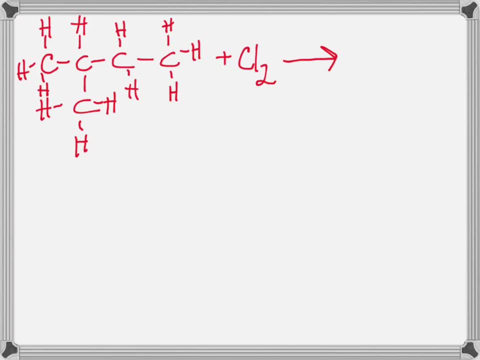 any of them is a possible product. So in this case there's many possible products. For instance, what we do know is remember this Cl2, if I just draw it a little bit differently- is really this: It's two chlorines bonded together by a covalent bond. 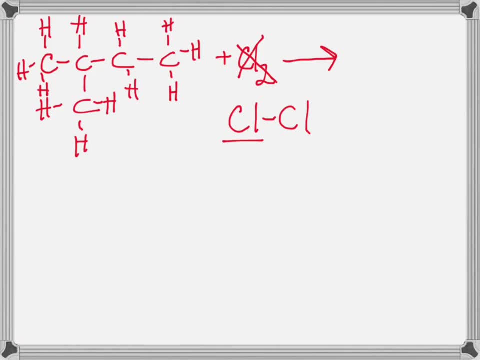 And we're going to take one of these chlorines and we're going to switch it with any of the hydrogens we want there And we're going to switch them. So, for instance, I could remove this one and remove that one and we're going to switch. 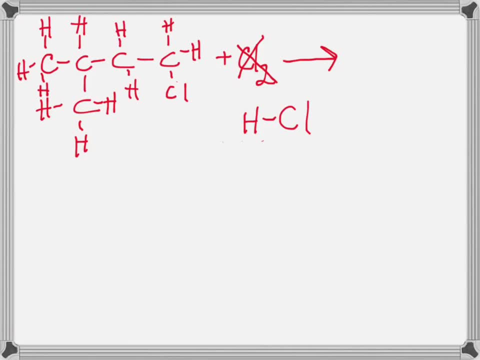 spots. So the chlorine will be there and the hydrogen will be there, right, That's one spot. I could have also switched it not to there, Just leave it there. And I could have switched it to this spot right here. That's possible. 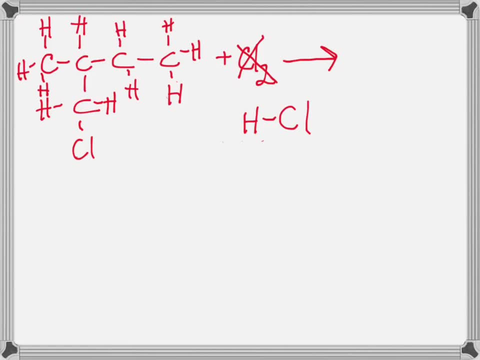 Or any of the spots, And that's a product of this reaction. Now, if we had a lot of chlorine in the reaction- and I didn't say whether there was a lot of chlorine or just a little chlorine- but if we just let the reaction go one time, this 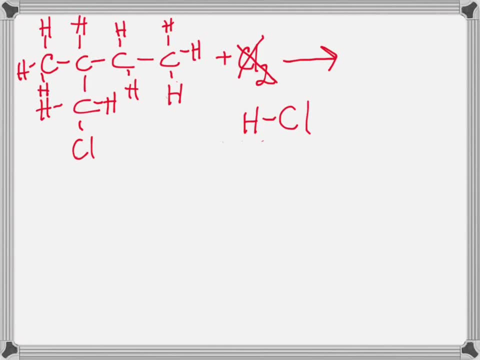 is a possible product If we added more chlorine. So if we added another molecule of chlorine, Right, I would switch one of these chlorines with one of these hydrogens. I'll pick this one right here. So let's go ahead and move this hydrogen and move this chlorine. 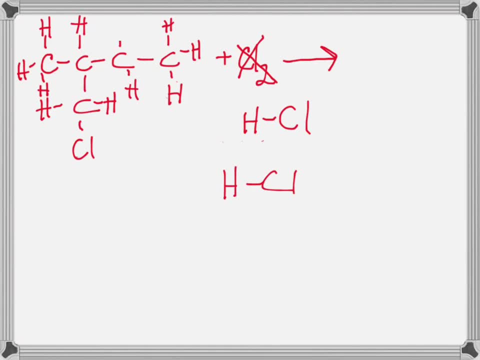 So the hydrogen will come down here and form HCl, and the chlorine will come up here and form that guy And we can continue to add chlorines until they are all completely full. All the hydrogens were removed and replaced by all chlorines. 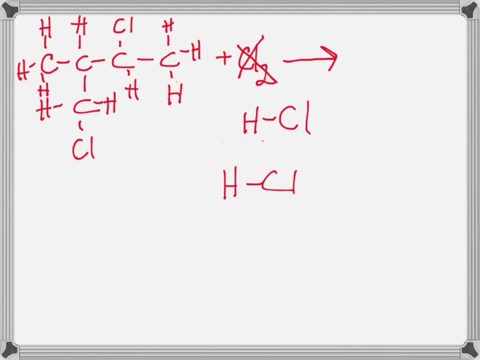 So there's a lot of different products here, for sure. But if the reaction just happens once- and we have, let me just go back to that- If the reaction just happens once and we get this and forget about, we won't worry. 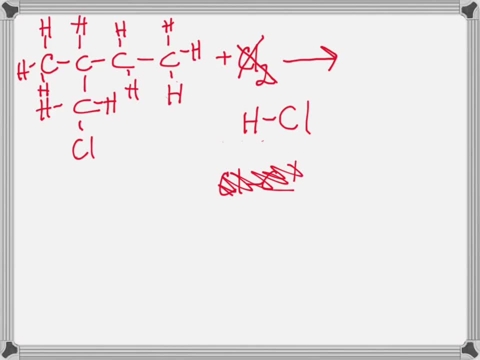 about that. So if the reaction just happens once, this is one possible product, but realize this chlorine could be in several spots to make a slightly different molecule. So there's more than one answer for this. Incorrect answers. But this would be one correct answer where you have two products. 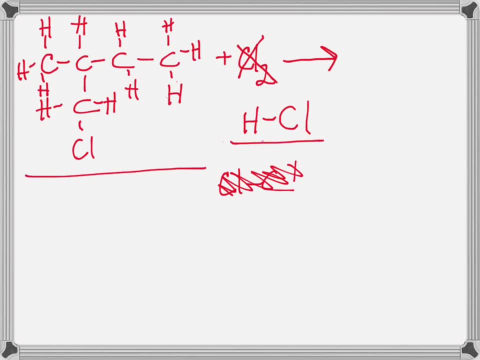 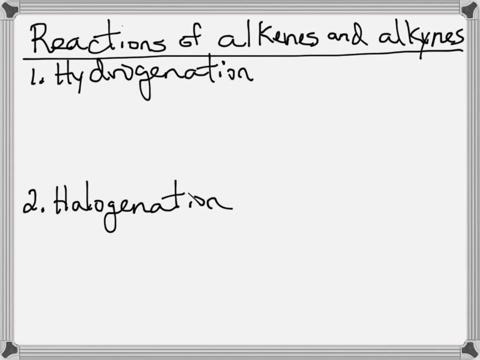 You have the alkane with a chlorine on it and you have the. no longer have a chlorine atom, you have a hydrogen chloride, the acid. Now, with alkenes and alkynes, we have four different reactions that can take place. 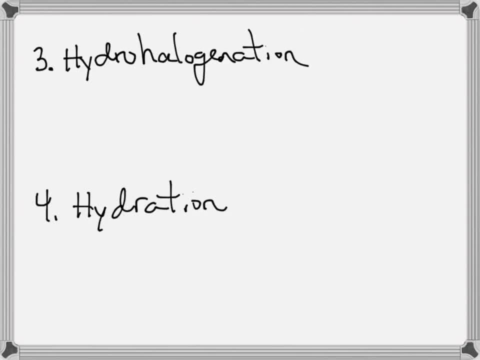 Hydrogenation, Halogenation, Hydrohalogenation, Hydrogenation And hydration. And a key thing to know about reactions of alkenes and alkynes. remember, alkenes have a carbon-carbon double bond and alkynes have a carbon-carbon triple bond. it is there that. 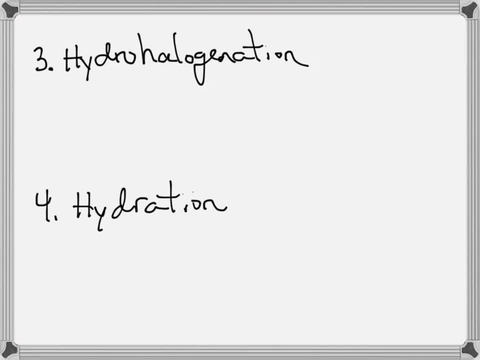 all the reactions occur. It occurs at the carbon-carbon double bond or at the carbon-carbon triple bond, It doesn't matter how big the molecules are. focus on that carbon-carbon double and carbon-carbon triple bond. That's where the changes are going to occur. 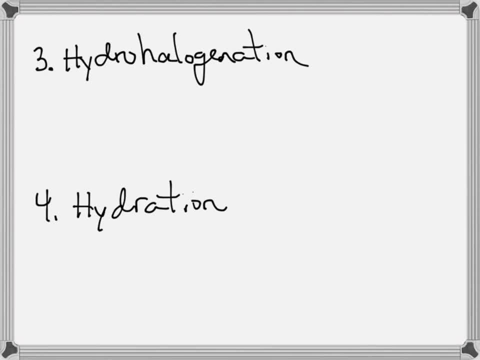 And with all these, what we're going to be doing is, you'll notice, we're breaking the double and triple bond and we're adding atoms to it. So we're going to take two things and combine them together to make one thing. 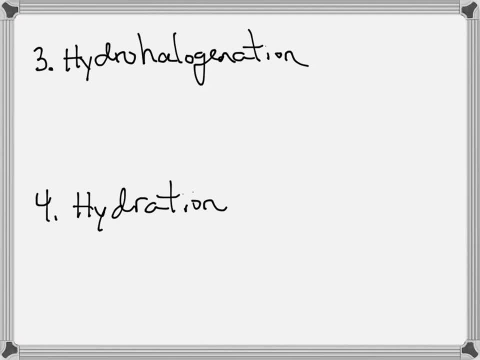 So it's an addition reaction Like three plus four equals seven. we took two things- three plus four, three and the four- and we combined them together to make the seven. In this case we're going to be taking two molecules. 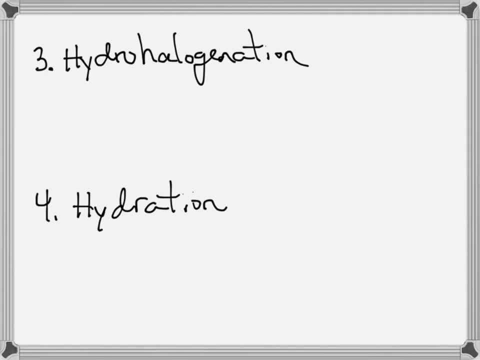 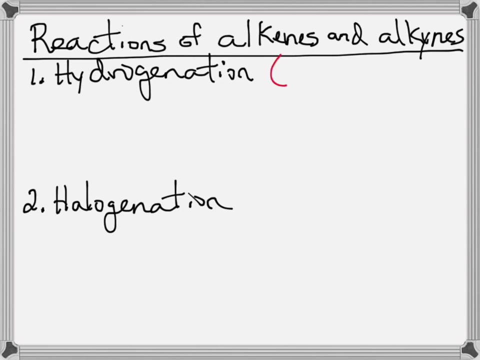 In each of these cases, we're going to be taking two molecules, combining them together to make one molecule. While combining them, we're breaking those double and triple bonds. So let's take a look at the first one, that's hydrogenation. 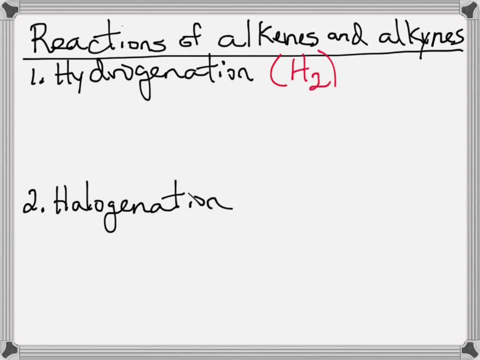 Hydrogenation is hydrogen. notice, that's part of the word. So we're dealing with hydrogen here again. just like chlorine and bromine and so forth, hydrogen exists in nature as H2, or H bound to H is another way to look at it. 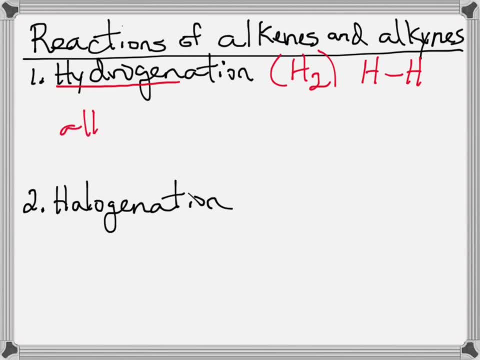 And what these can do is: we can take any alkene or alkyne, we add the hydrogen to it and what we're going to get is an alkane. So by doing this, the alkene will become an alkane. the alkyne will lose one of the 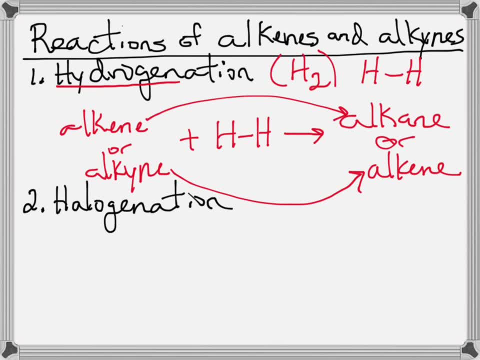 bonds. it'll go from three bonds to two bonds. And notice, with the alkene we go from a carbon-carbon double bond to a carbon-carbon single bond. We're going to break that one of those bonds In halogenation. again we start with an alkene or an alkyne. 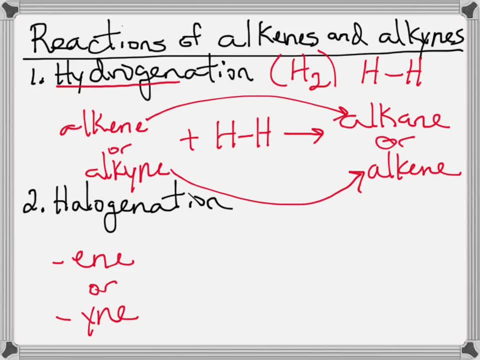 And I'm just going to break that one. I'm just abbreviating there. it's the same as on the first one. Now, halogenation: we just learned just a moment ago in all the halogens F2, Cl2, Br2.. 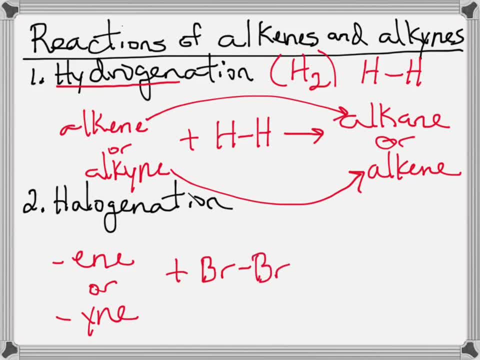 So we can take any halogen we want, and just as an example I'll use Br. And what do we get there is we get a dibromo. so two bromines on an alkane or dibromo, two bromones on an alkene. 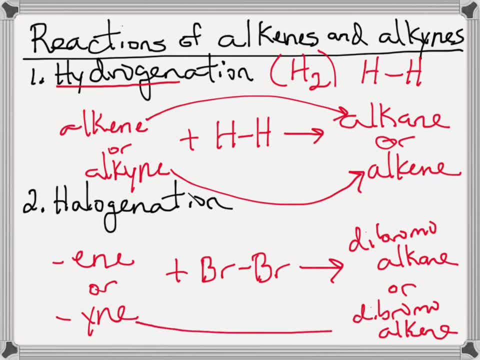 Again, the alkyne, which is a carbon-carbon triple bond, will be removed and one of those bonds can be broken to make an alkene with a carbon-carbon double bond. Or we take a carbon-carbon double bond and we break one of those bonds to make a carbon-carbon. 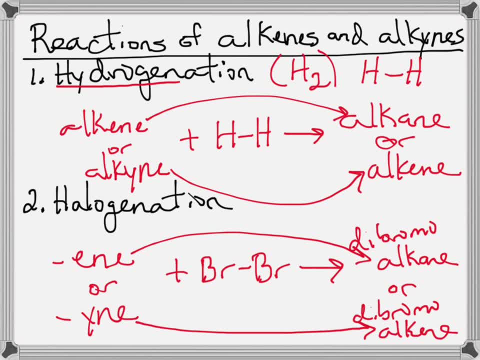 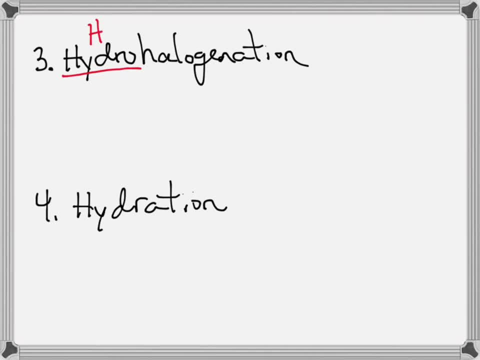 single bond and the bromo groups are added to it. Hydrohalogenation- Notice hydro, that's H, and we know what halogens are, and so these would be things like HBr or HCl or Hi or HF- any of those- because it has a hydrogen and a halogen. 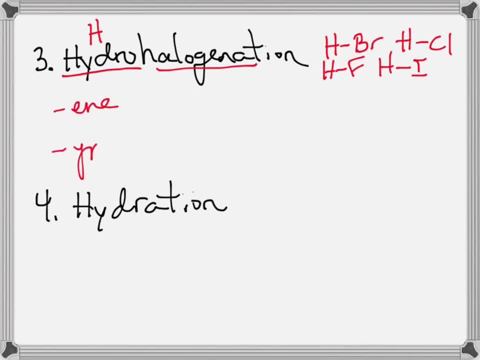 And it's the same. We can take our alkenes and alkynes plus again, I can use any of them, but that's an example of one, And so in this case I would get a chloroalkane, so an alkane with a chloro group on it, or 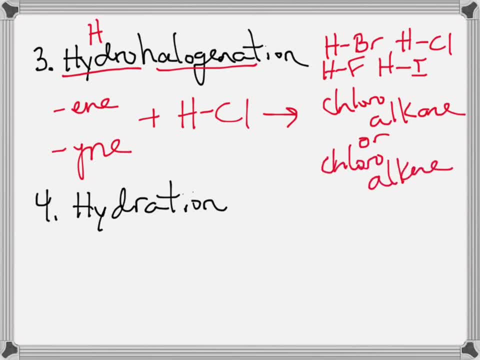 a chloro with an alkene, depending on if I started with an alkyne or an alkene In a hydration reaction. hydration we can recognize as water and again we can take our alkene or alkynes. We can add a molecule. 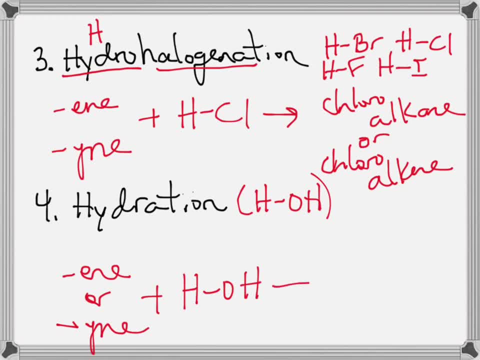 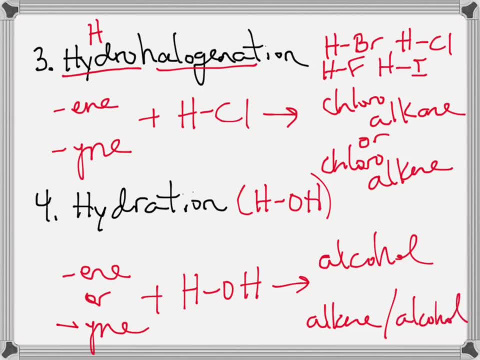 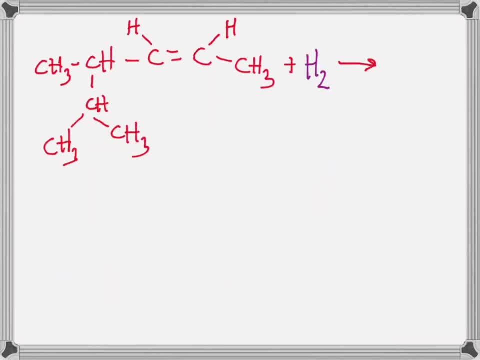 with an alcohol group as well on it. so it's sort of a mixture And I'll give you a couple of examples of each of these. an example of each of these. So here's one. So go ahead and give this one a try, based on what we just talked about, and see if you. 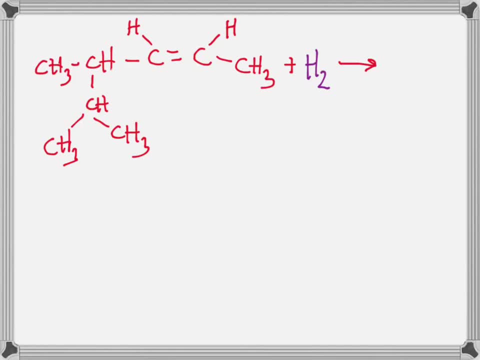 can come up with the product of this reaction. When you think you have the product, come on back and we'll chat about it. So in this reaction we first take a look at what we have and notice we have an alkene right here, right. 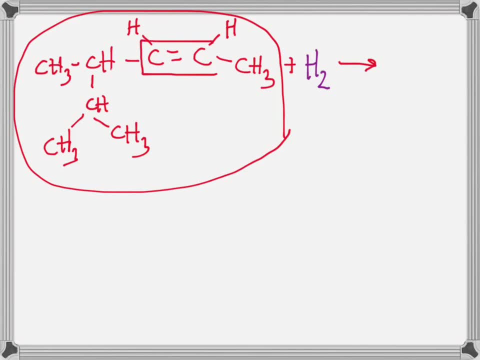 You can see it's an alkene, because I see this carbon-carbon double bond right there. so I know I have an alkene. There's a lot of stuff hanging on it, but nonetheless that's an alkene. and then I'm 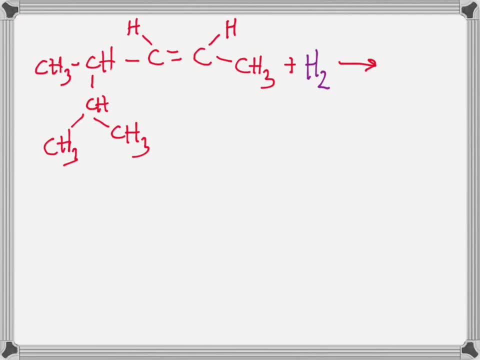 adding hydrogen to it. So this is a hydrogenation reaction because I'm adding hydrogen to it and, remember, this is an addition reaction. so we're going to take this alkene and add on the hydrogens. And I told you, when you do this, focus on that carbon-carbon multiple bond, that carbon-carbon. 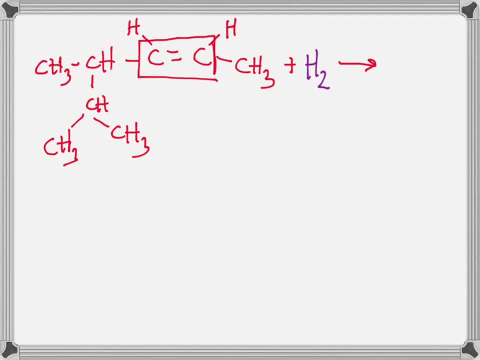 double bond in this case. so we're going to focus everything right here Now because we're adding things to it. we're not going to subtract anything. So the things currently hanging on the carbon, those two carbons involved in the double bond, 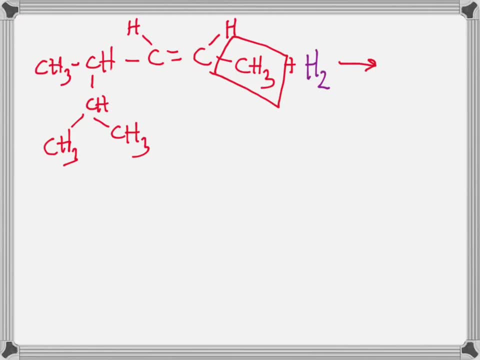 meaning this methyl group. that will still be there when we're done. This will still be there when we're done, because, remember, we're adding, we're not subtracting. This will be there when we're done, and all of this will be there when we're done. 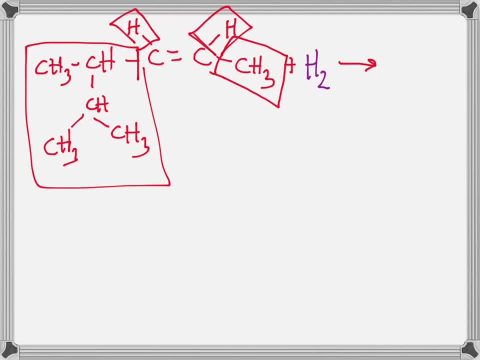 So really we can just kind of in our heads, just kind of remove that from our brain for a moment, at least mentally, and we're going to just focus on that carbon-carbon double bond that we did not square up there. Now I'm going to remove the squares just to clean this up a little bit, but just mentally. 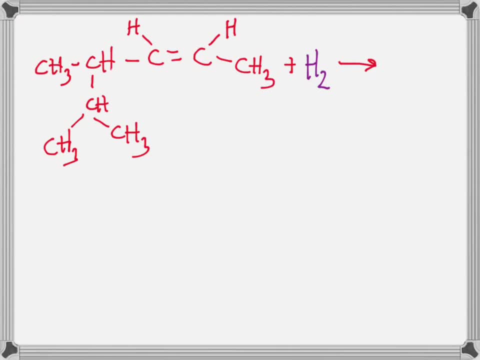 So I'm going to focus just on that carbon-carbon double bond, and what happens is that we're going to add it, So let's take these hydrogens now. remember, this hydrogen is really that, and we're going to float it on over to here just so we get it a little bit closer. 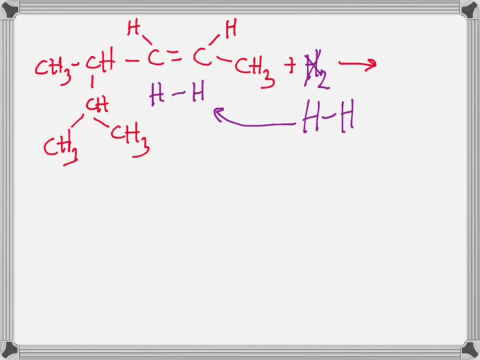 So I'm going to put them right here. so we're going to line it up and all we're going to do is we're going to break that carbon, We're going to break that carbon-carbon double bond and we're going to break this hydrogen-hydrogen. 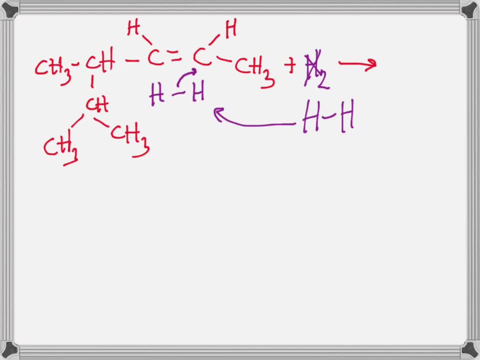 bond. So I'm going to move this bond to here, move this bond to here, essentially, and we're going to create new bonds. Let me go ahead and erase the old bonds and let's put the new bonds in. and the color. 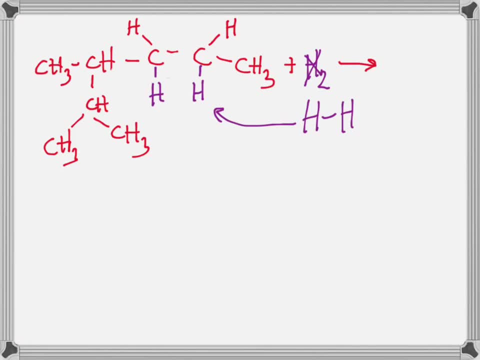 here, doesn't matter, I just happen to have a purple pen on me. that's what it is. So now you can see the new hydrogen-hydrogen bond. So we've created two new hydrogens, we've added on the two new hydrogens and we now 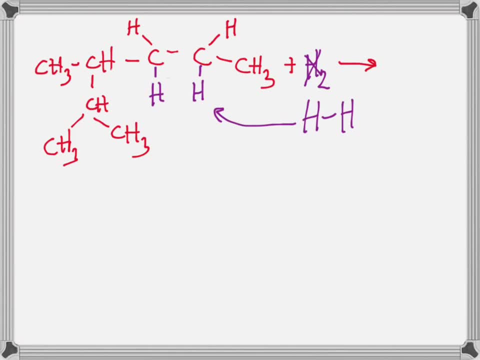 have a carbon-carbon single bond where we used to have a carbon-carbon double bond Here. now we have an alkane, so we've made an alkane in this process. What's the other product? Well, there is no other product. we added all of that one. we added all of this to the alkene. 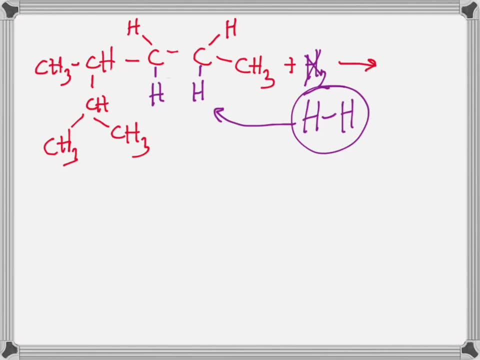 to form the alkane, And so that's our product. so we have an alkane as a product, and the two new hydrogens are added on. So let's try this one, here's another one. So go ahead and determine what the product of this reaction is. 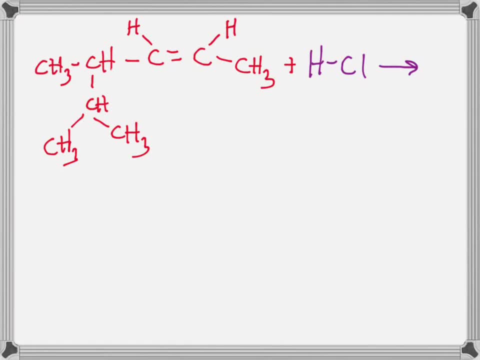 So go ahead and pause the video, then come on back when you're ready and we'll chat about it. So in this one again, I see I have an alkene shown in red here, the same one we had in the previous reaction. 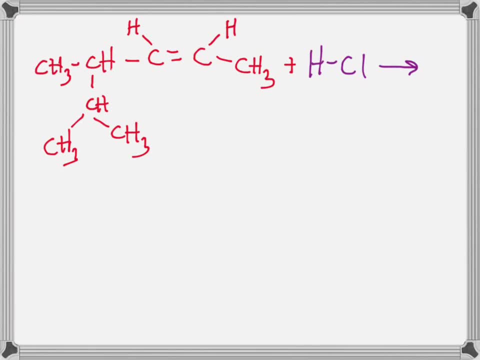 But this time we don't have a hydrogen molecule, we have a hydrohalogen. So this is a hydrohalogenation reaction, But you'll see, it's pretty much the same as the hydrogenation reaction with the hydrogen atom. Again, let's just focus on where the reaction is going to occur and the reaction is going. 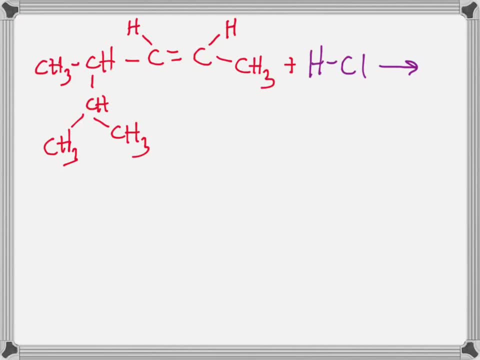 to occur right around that carbon-carbon double bond. So let's go ahead and take this hydrohalogen and we're going to move it on over to here. So we're going to remove it from there, we're just going to slide it on over here to get. 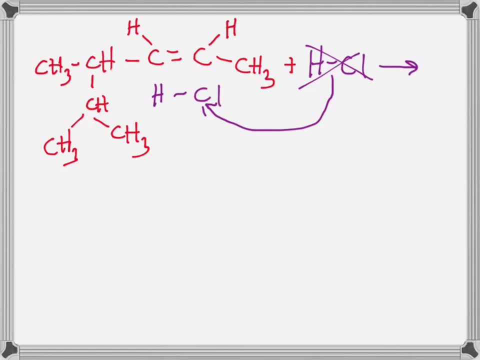 it close to where it wants to go. And then we're going to go ahead and start breaking some bonds. We know we're going to break the carbon-carbon double bond- at least one of them- and make it a single bond. So we'll move this bond to here and we'll move the bond between the hydrogen and the. 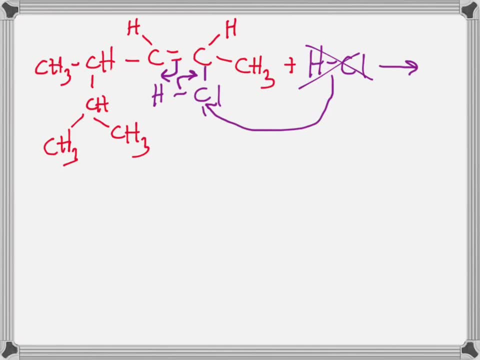 chloride over to here to form two new bonds. And let me go ahead and erase what is now gone And notice here again: now what we have formed is the product, So it's a single molecule, as the product Notice. we took the alkene, we took the hydrogen halide and we just combined them together. 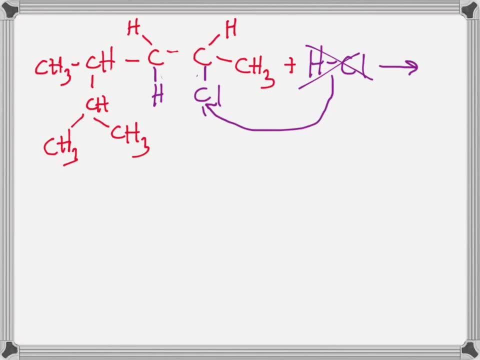 to form one molecule. So there's only one product And we bound. we now have an alkane as our product, and the alkane does have a chloride on it. Now it doesn't matter which way I put the hydrogen and the chloride on. 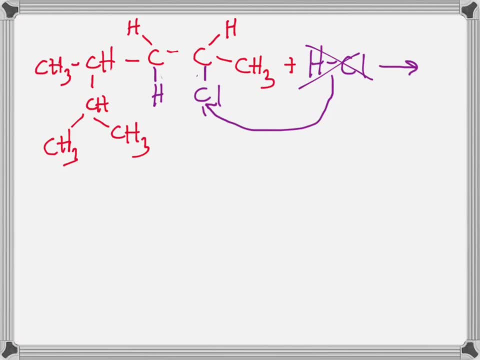 I could have done it the way I did it here. Or Let me erase a few things here and let's say, instead of attacking like this, I put the hydrogen here and the chloride over here. That would move the chloride to a different carbon, so it makes a different product. 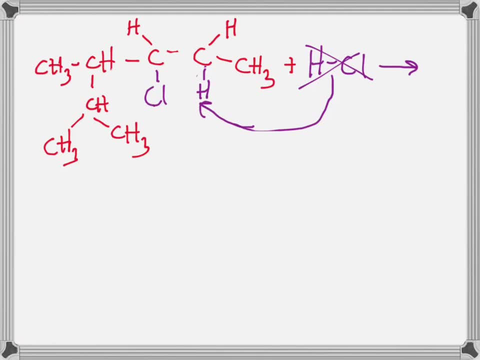 So although we add two things together to make one molecule, we could have made a couple of different molecules: either the chloride on this carbon- whoops- either the chloride on this carbon or the chloride on this carbon. Either way, we still made an alkane with one chlorine atom on it. 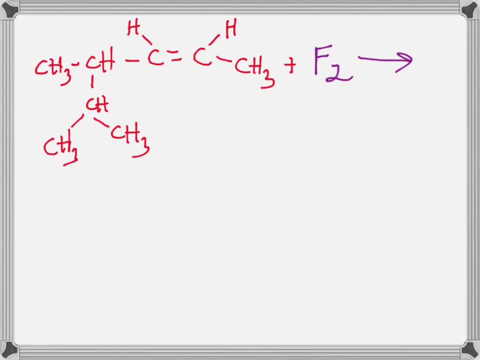 So here's another one to try. You can go ahead and give this one a try, determine what the product is, and then come on back and we can chat about it. So again, we see that we have an alkene here with a carbon-carbon double bond, and so we 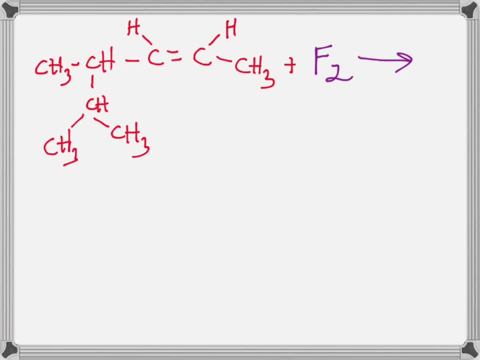 know that we're probably going to be going after that carbon-carbon double bond. That's where we're going to attack and that's where the reaction's going to occur. It doesn't really matter what else is on. Notice that in all these reactions, we don't really care what else is on the carbon-carbon. 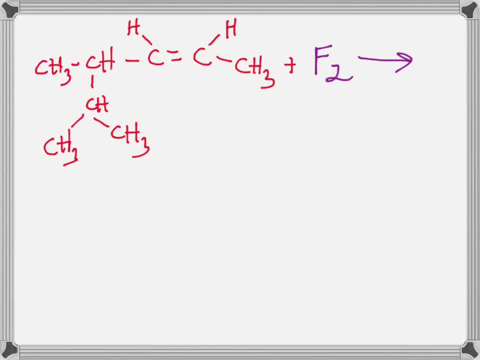 attached to the carbons of the carbon-carbon double bond. Those don't get changed in any way. Here we have a fluorine fluoride ion And here we have an alkene. Here we have an alkene. Here we have an alkene. 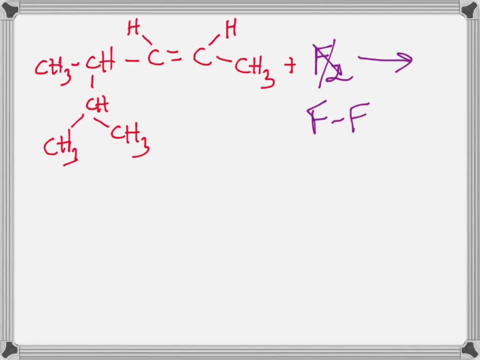 And, I'm sorry, fluoride- And we have- we can redraw it like that, where it's two fluorines connected by a covalent bond And we're going to move that guy right on over to here and we're going to have the 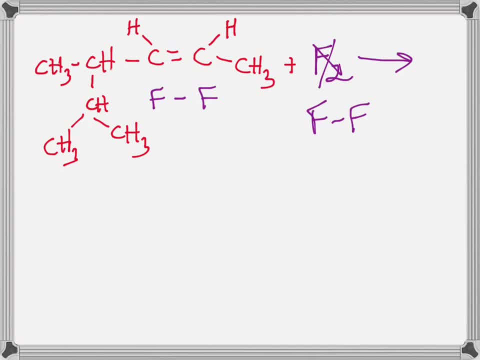 reaction go. And in this case again, we're going to move one of the carbon-carbon double bonds on down, the bond connected to the two fluorines over here. So we move those two. So let me now remove what is now gone after moving those electrons. 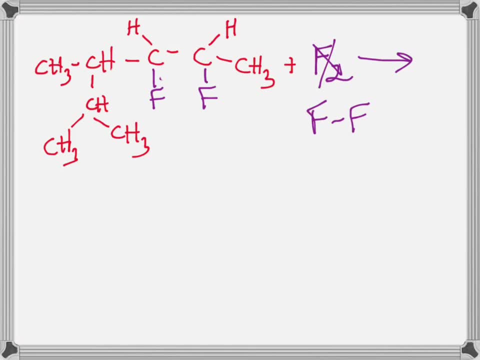 And we're going to move that guy to a different spot And we get that guy. And again, since the two fluorines are the same, it doesn't really matter which way they connect to the carbons. There's always going to be one fluorine on one and one fluorine on the other carbon. 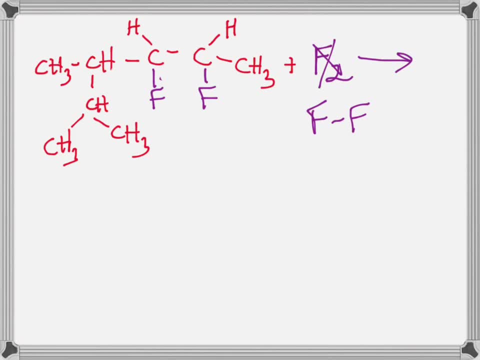 And so there's one product in this reaction. again, we've added two things together to make one thing, And so that's our product. Notice that it was an alkene. It lost a double bond and went to a single bond, and so now it becomes an alkane with. 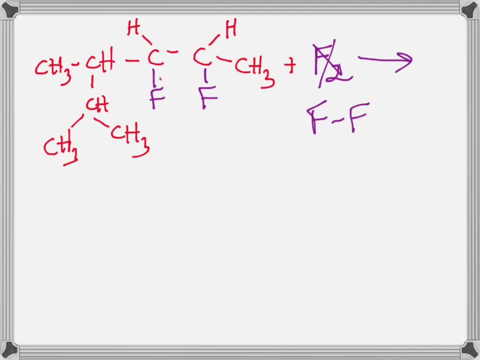 two fluorines on it Or two halogens on the molecule. Okay, we'll do one more. Go ahead and determine what the product of this reaction is. Just put the arrow over here. Determine what the product of this is. When you think you've determined what the product is, come on back and we'll chat about. 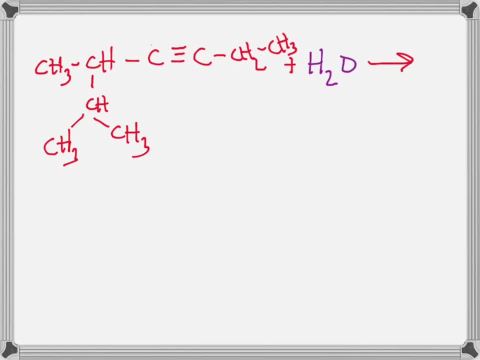 it. So in this one now, this is a little bit different. this time. Now we don't have an alkene, We have an alkyne, Notice the carbon-carbon triple bond in there. But it doesn't change our strategy at all. 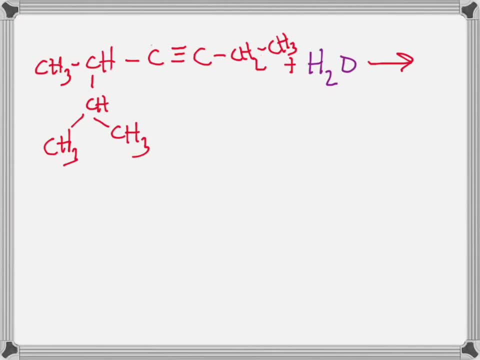 It's a little bit different, It looks a little bit different, but keep the method of what you're doing the same. We're also going to be adding a molecule of water, So this is a hydration reaction, because we're adding water, Water's hydration. 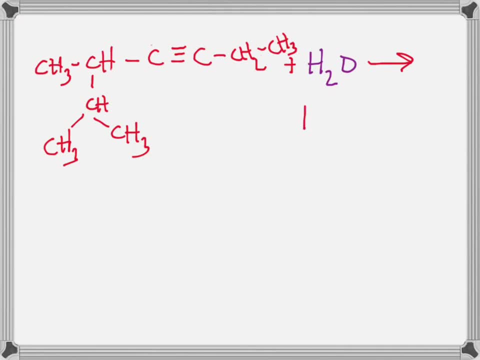 And so we're going to change this molecule, this water molecule, to make it look ready to add on to our alkyne. So again, we're going to be adding it on. Water likes to break apart. Notice, there's not two atoms here, but three atoms. 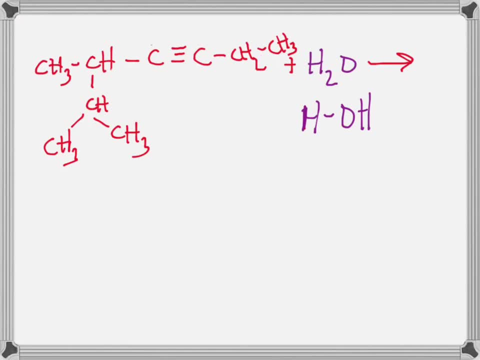 But it likes to break apart between the oxygen and one of the hydrogens to form a hydrogen and a hydroxyl group, And so we're going to go ahead and move that on over to here. So we'll put a hydrogen here, bond it to a hydroxyl group here. 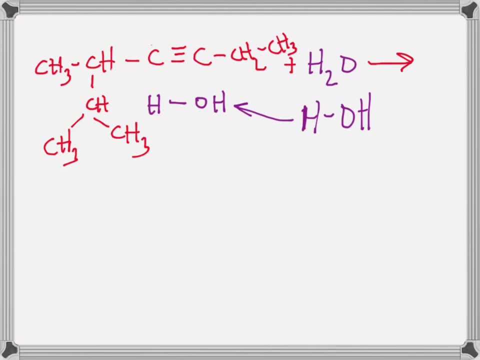 But at this point again, we just do it the same way we've been doing. It doesn't matter that it's an OH or an F or whatever. We're just going to do it the same way we've been doing. It doesn't matter that it's an OH or an F or whatever. 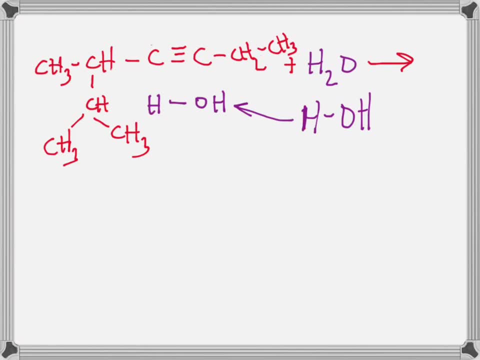 This is what we're just going to work with, And we're going to do the same thing as we've done before: We're going to move one of the bonds of the triple bond, so not two of them, just one of them. 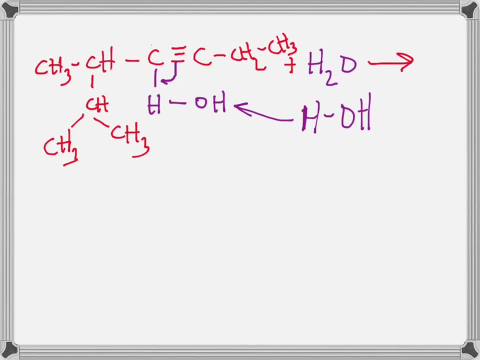 We're going to move it on down to here, as we've done before, And we'll move the bond connecting the hydrogen and the oxygen on up to here to go there. Let me go ahead and erase what is now gone after we move those electrons. 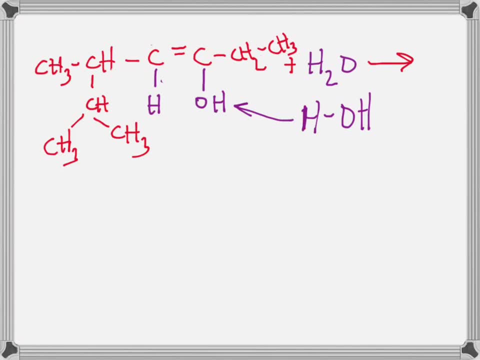 And that is what we get. Okay, We get that molecule right there. Notice, this is got a carbon-carbon double bond, so it looks kind of like an alkene, But it also has an OH group, so it also has an alcohol. look to it. 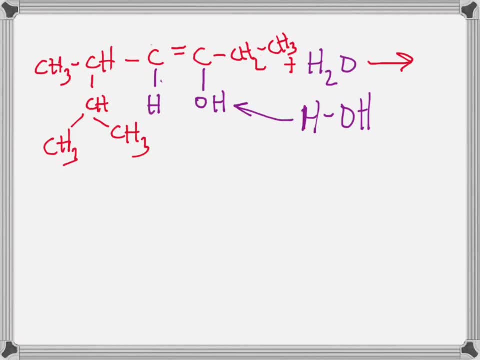 So it's basically an alcohol and an alkene. Now we could have put that on in the opposite direction, meaning I could have not ended up with a hydroxyl group. I could have put it on the one carbon but put it on the other carbon. 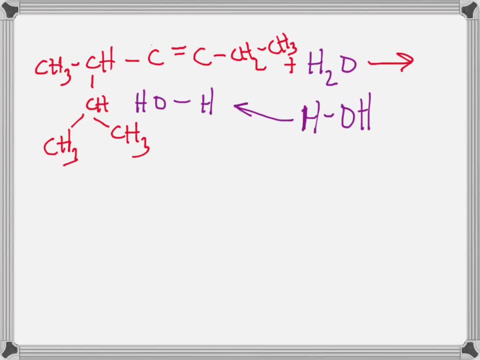 So we could have basically had this: look, Let me get my three bonds back. There's my three bonds And, just as before, because the two atoms that are connecting to the carbons of the triple and double bond are different, there's two different ways in which it could go on. 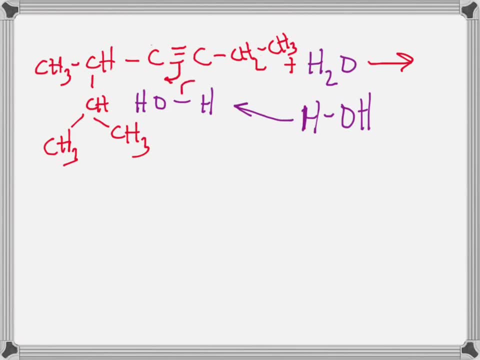 But still the same thing happens. We move one bond down to here, one bond up to here to form these two bonds, and let's get rid of what has now gone. It's been moved because of that reaction and we get that. 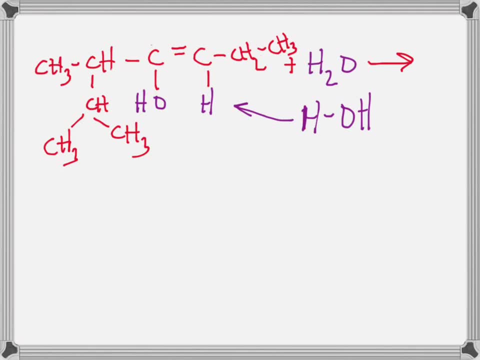 Notice: in this case this is also a possible product, but notice: in this case the OH group is now on a different carbon than it was previously. Now, if there was enough water around- because now we have an alkene- it could undergo the. 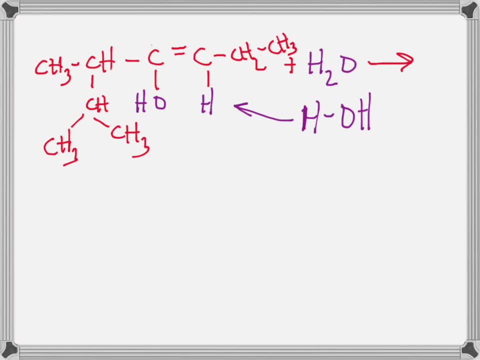 reaction again, And so we could actually have another molecule of water. I don't know how much space I have, but let's take another molecule of water And in a second reaction, because there's an alkene still there. oops, I'm having. 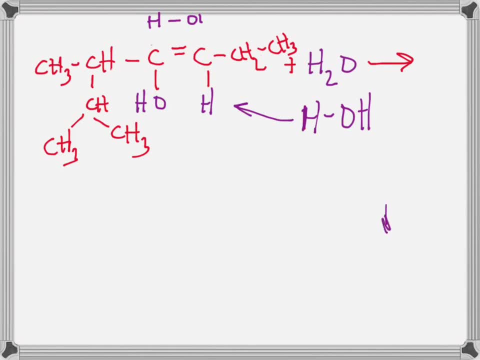 trouble getting that. there we go. it's not wanting to do it. I don't know why, But you can see those two lines there. that's supposed to be an H. it's just not wanting to connect for some reason. Oh, there we go. 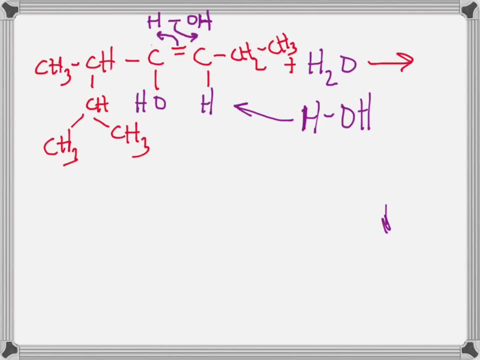 And one of the bonds will move to here. one of the bonds will move to here, So we'll connect those. Let's erase what's in between or what was lost in that reaction, And we get that. And that bond should be connected to the oxygen, not the hydrogen. 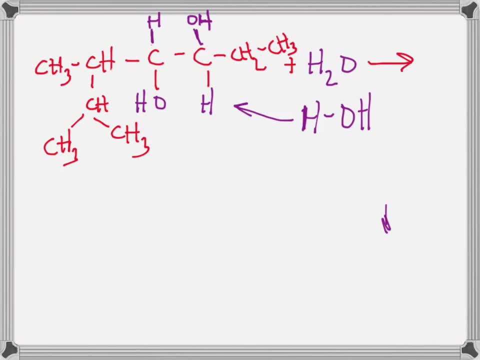 And so we get that And again that one could have gone on either way, so the OH group could have ended up on the carbon it's showing it's ended up on or could have ended up on this carbon, So it could have gone either way. 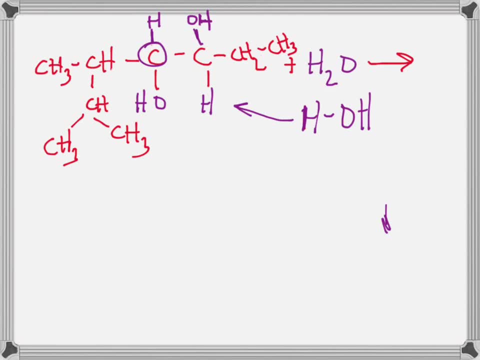 So in the end, Because this reaction happened twice, we could have the OHs on the same carbon or different carbons. Both are possible and both are correct in terms of being able to form, So both will form. they just might not form in the right. the same amounts. 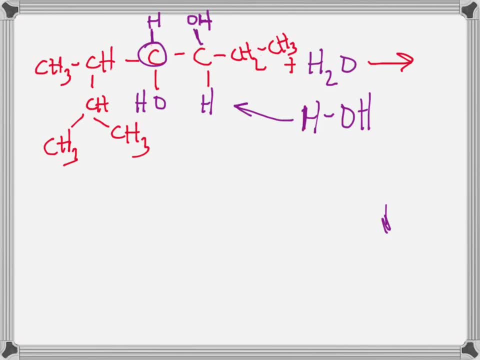 But nonetheless, both will form. So this is a hydration reaction and this reaction I showed you what it looks like with a triple bond and a double bond because we did both. So if you started with a double bond, the same thing would happen: we'd add a molecule. 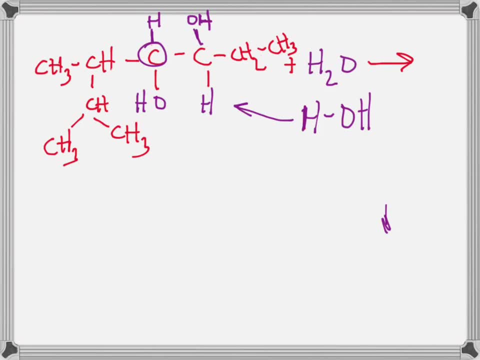 of water, We'd make an alkane with a hydroxyl group on it, which is essentially an alcohol.